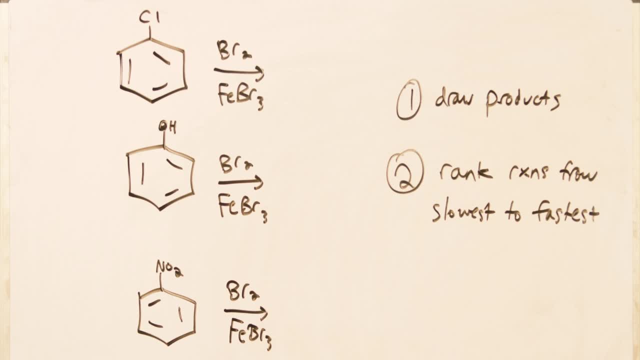 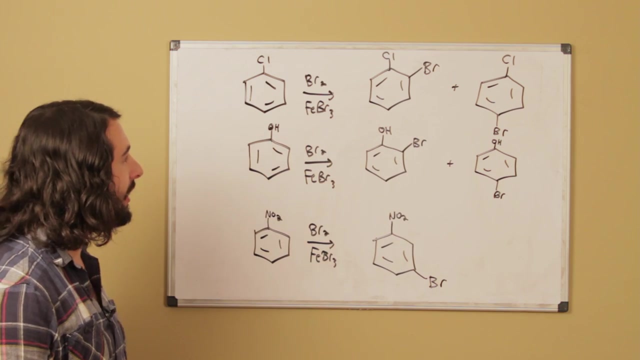 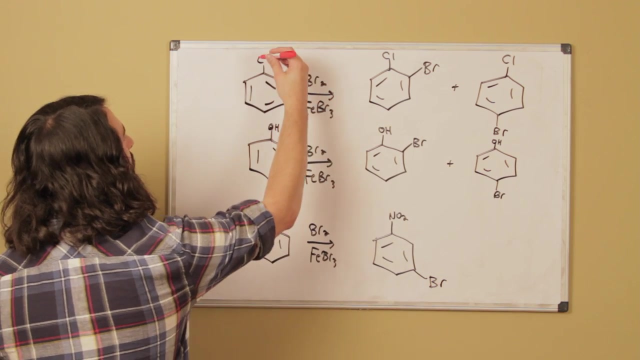 okay, so I've gone ahead and drawn the correct products for these brominations. now the key to drawing these products is understanding the directing capabilities of these functional groups. so a chloro group, any halogen, is an ortho para director, so we're going to get a combination of 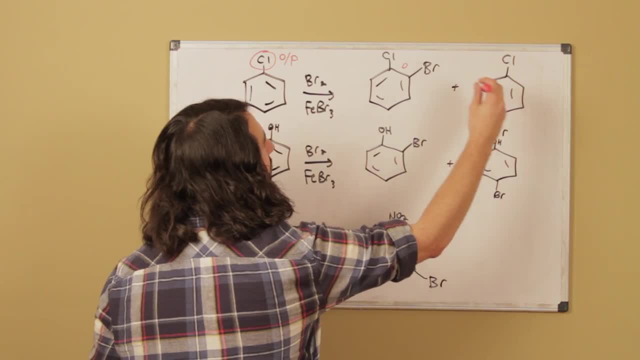 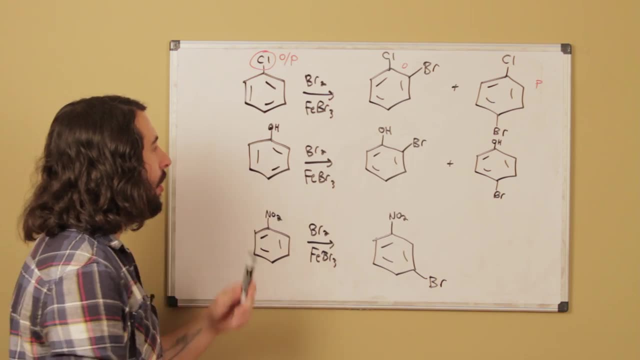 ortho and para products. so this is the ortho product, this is the para product. right and so same over here. with this phenol, the hydroxyl group is also going to be an ortho para director. so here is our ortho substituted product, here is our. 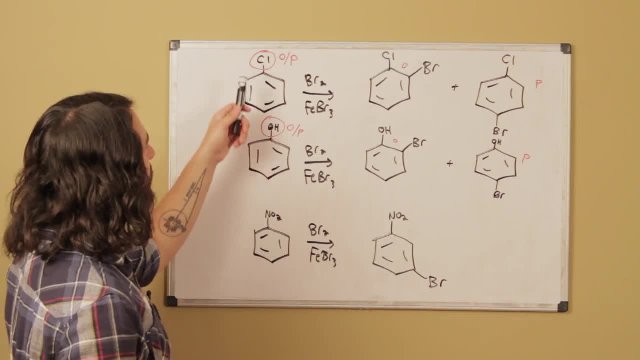 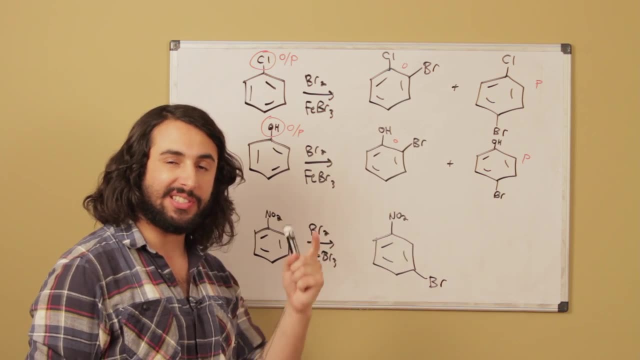 para substituted product. now, these are both ortho para directors, even though the halogens are electron withdrawing. typically, electron withdrawing groups are meta directors, but remember that halogens is that one exception. halogens are still ortho para directors and hydroxyl groups are ortho. 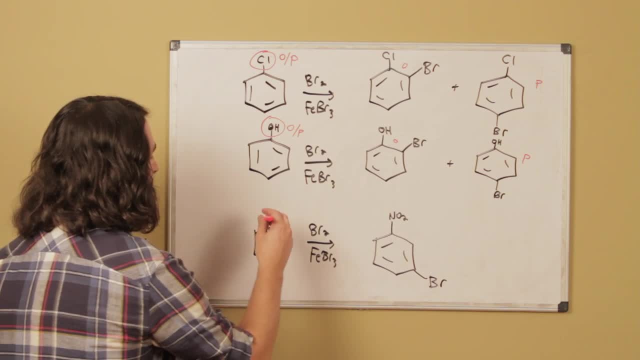 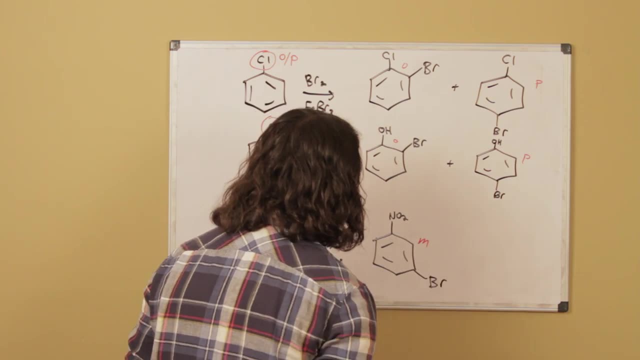 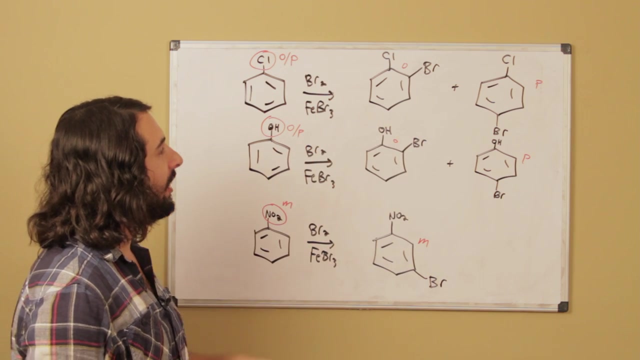 para directors, because they're electron donating, and then, lastly, the nitro group. the nitro group, because it is strongly electron withdrawing, that is going to be a meta director, so we do get the meta substituted product. so, number one, we do want to talk about the regioselectivity of these in order to be able to draw the 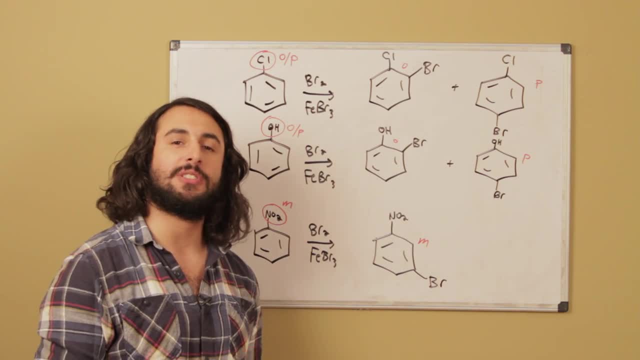 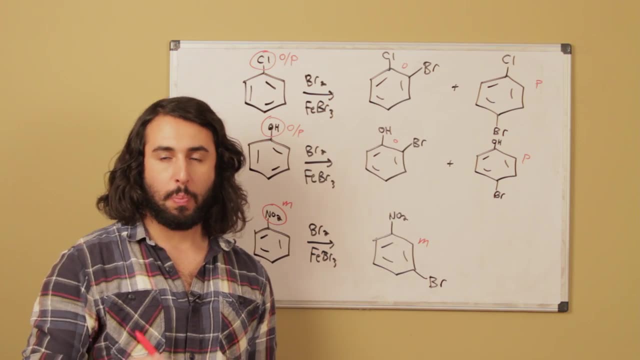 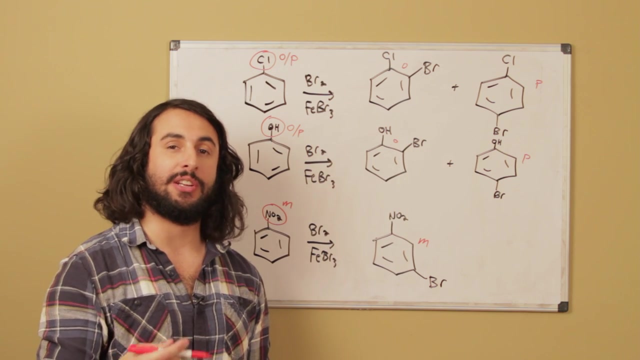 the dominant products. but then we also want to talk about kinetics. we want to talk about the speed of the reaction. see which ones are going to go the fastest. well, we know that the intermediate in a electrophilic aromatic substitution reaction is an arenium ion intermediate. it is a positively charged intermediate. 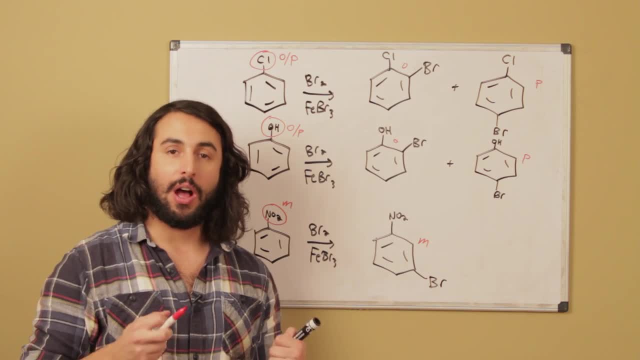 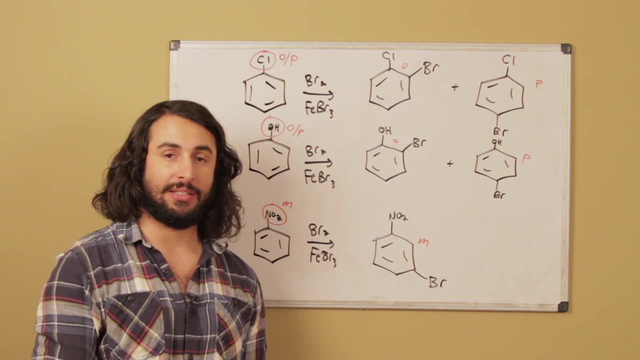 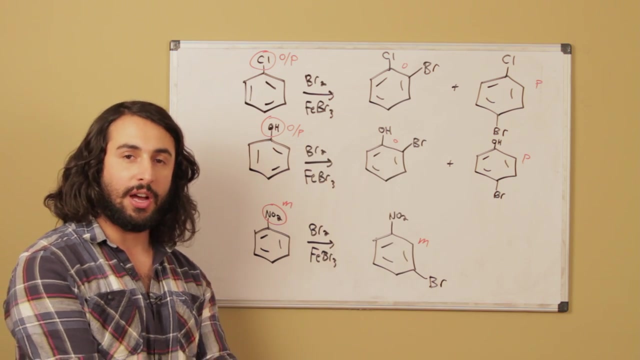 so when we have electron withdrawing groups that are already on the ring, they're going to further destabilize the arenium ion intermediate, and so they're going to make the reaction proceed more slowly. now, here, the nitro group is the strongest deactivator. it's the strongest electron withdrawing group, so it is. 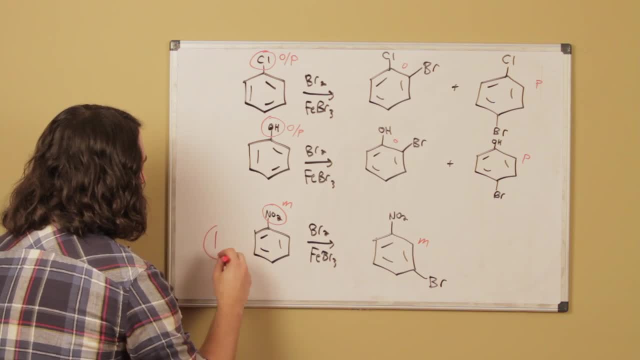 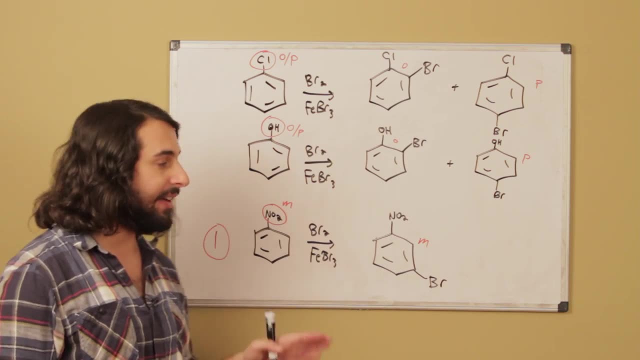 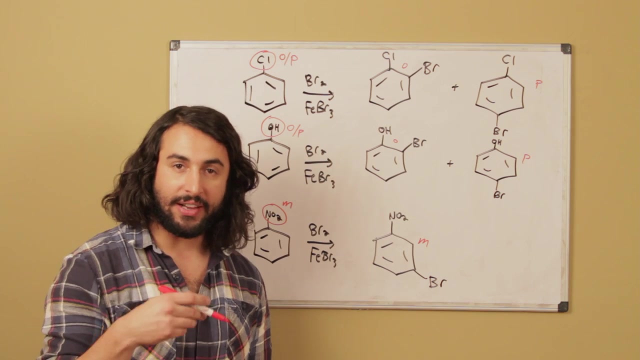 going to destabilize the intermediate the most and therefore it will be the slowest reaction. now the halogens over here, halogens are also withdrawing, not by resonance, the way that the nitro groups do, but actually by induction, just by the, the electronegativity of that carbon halogen bond. so those